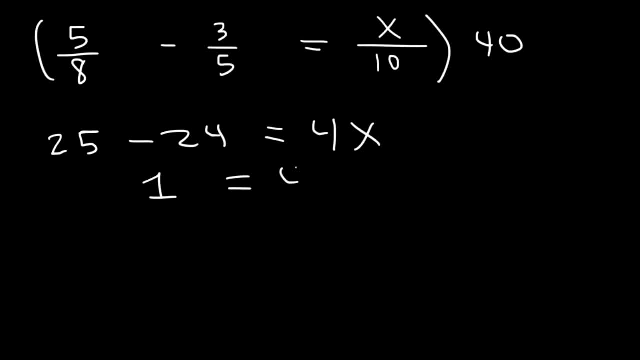 25 minus 24 is 1, and so x is equal to 1 fourth. So that's the answer. Here's the next problem: x plus 8 over x is equal to 6.. Feel free to pause the video and work on this example. 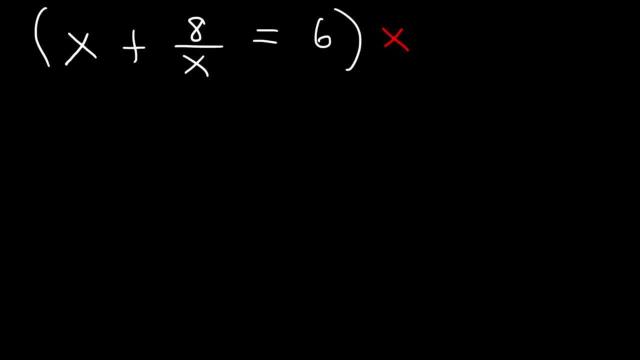 So what we're going to do in this problem? we're going to multiply both sides by x. So x times x is x squared, and then 8 over x times x, the x variables will cancel, it's just going to be 8, and 6 times x is 6x. 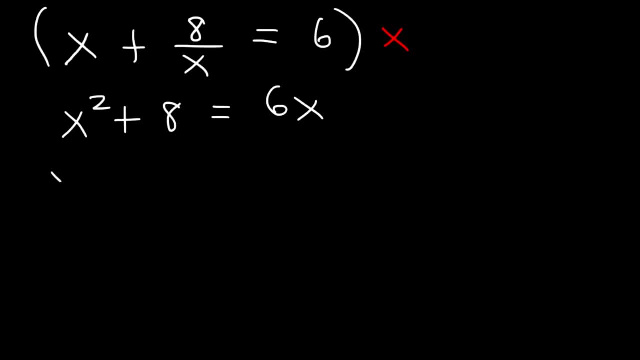 Now let's move the 6x from the right side to the left side. On the right side it's positive 6x, but on the left side it's going to be negative. Now we can factor it: What two numbers multiply to 8 but add up to negative 6?? 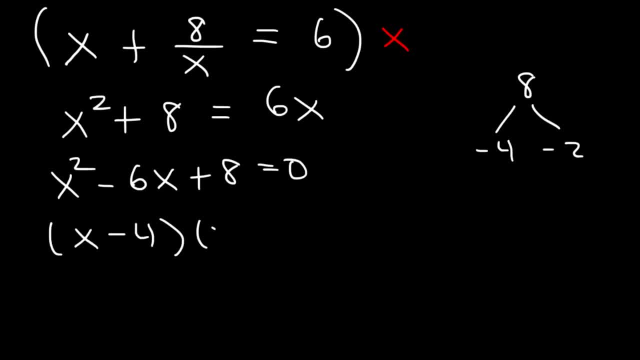 This is negative 4 and 2.. So it's x minus 4 times x minus 2.. And so we can clearly see that x is equal to positive 4 and positive 2.. So that's it. Here's the next one. 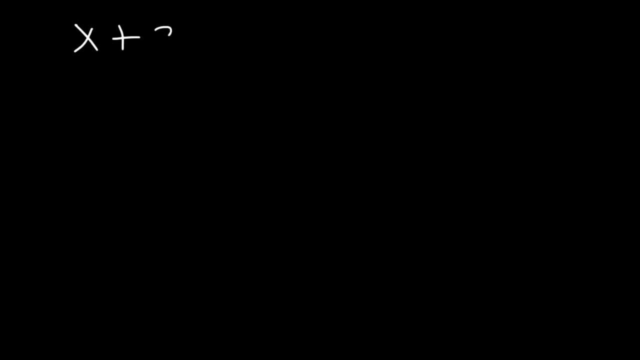 x plus 3.. 3. Divided by x minus 3. Let's say that's equal to 12 over 3.. Whenever you have two fractions separated by an equal sign, what you want to do is you want to cross multiply. 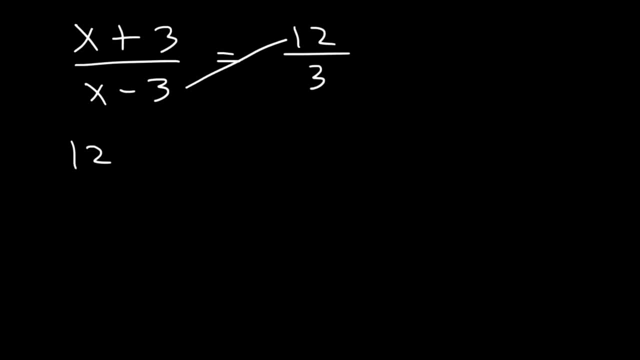 So 12 times x minus 3 is 12x minus 36.. And 3 times x plus 3, that's 3x plus 9.. Now let's subtract x, 3x plus 9.. 3x plus 9.. 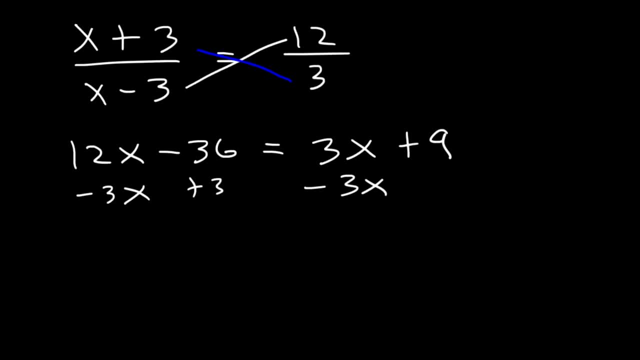 Let's subtract both sides by 3x And let's add 36 to both sides. 12x minus 3x is 9x. 9 plus 36 is 45.. And 45 divided by 9 is 5.. 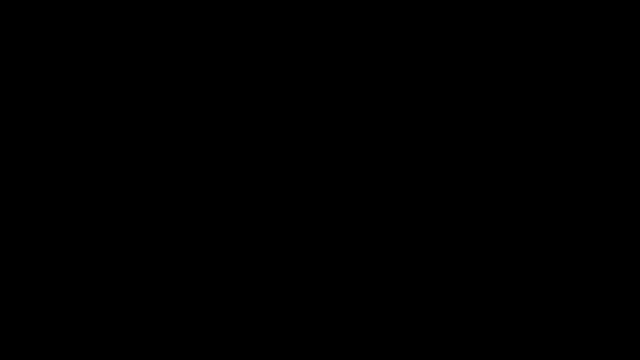 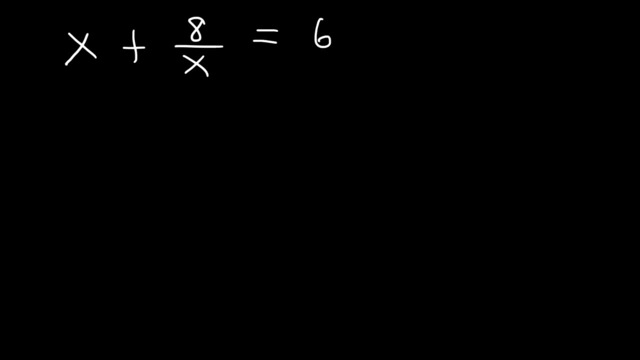 Feel free to pause the video and work on this example. So what we're going to do in this problem, we're going to multiply both sides by x. So x times x is x squared, and then 8 over x times x, the x variables will cancel, it's just going to be 8, and 6 times x is 6x. Now let's move the 6x from the right side to the left side. On the right side it's positive 6x, but on the left side it's going to be negative. 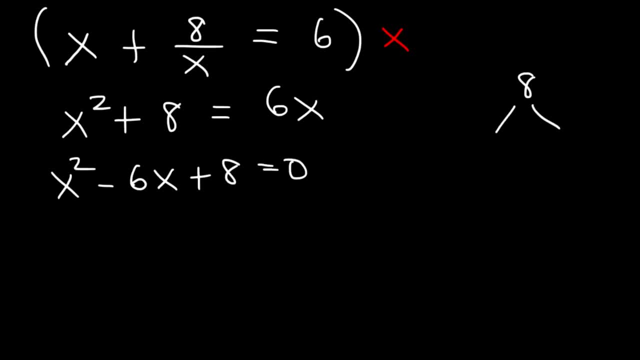 Now we can factor it. What two numbers multiply to 8 but add up to negative 6? This is negative 4 and 2. So it's x minus 4 times x minus 2. 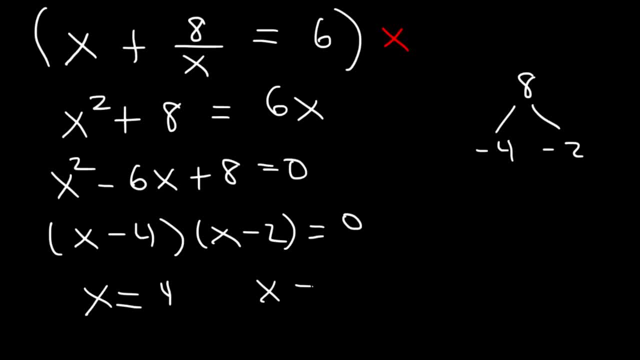 And so we can clearly see that x is equal to positive 4 and positive 2. So that's it. 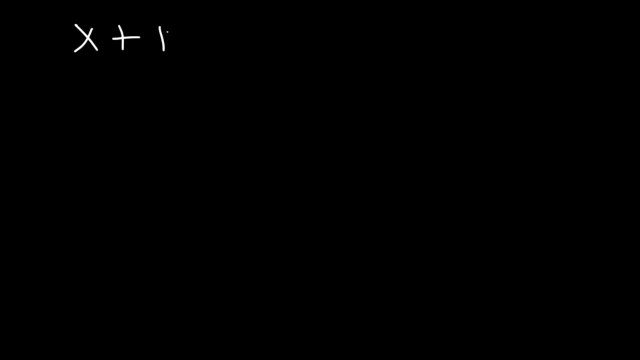 Here's the next one. x plus 3. 3. 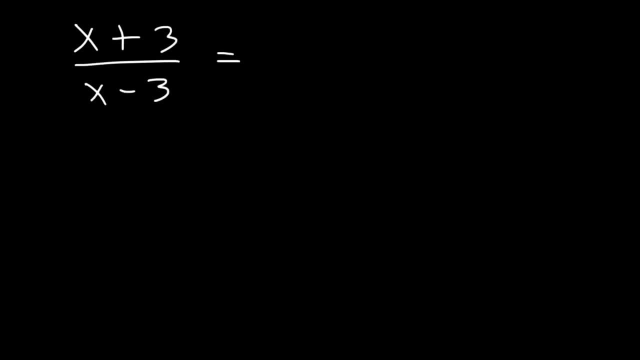 Divided by x minus 3. Let's say that's equal to 12 over 3. Whenever you have two fractions separated by an equal sign, what you want to do is you want to cross multiply. 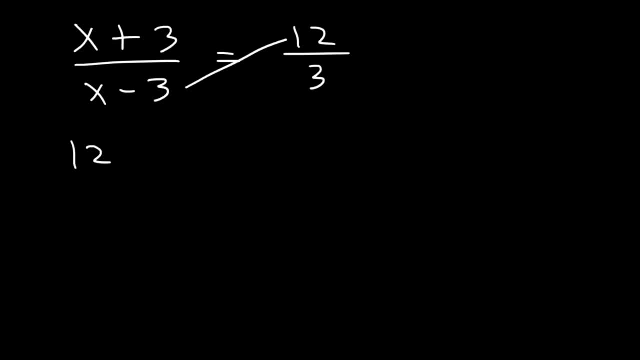 So 12 times x minus 3 is 12x minus 36. And 3 times x plus 3, that's 3x plus 9. Now let's subtract x. 3x plus 9. 3x plus 9. 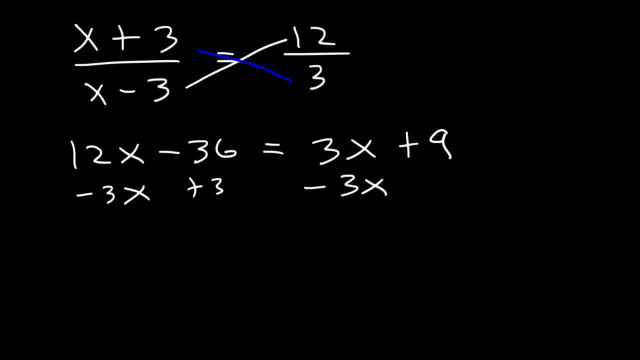 Let's subtract both sides by 3x and let's add 36 to both sides. 12x minus 3x is 9x. 9 plus 36 is 45. And 45 divided by 9 is 5. So x is equal to 5. Try this one. 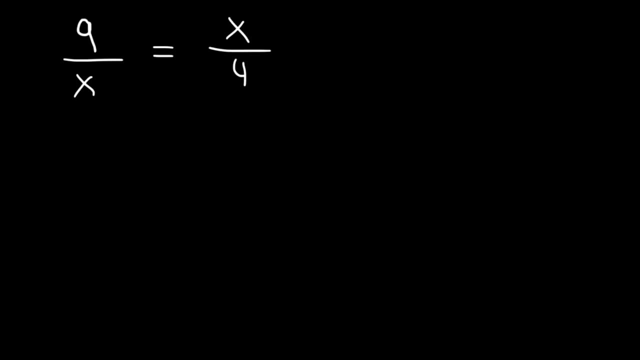 9 divided by x is x over 4. 9 divided by x is x over 4. So, once again, we have two fractions separated by an equal sign. 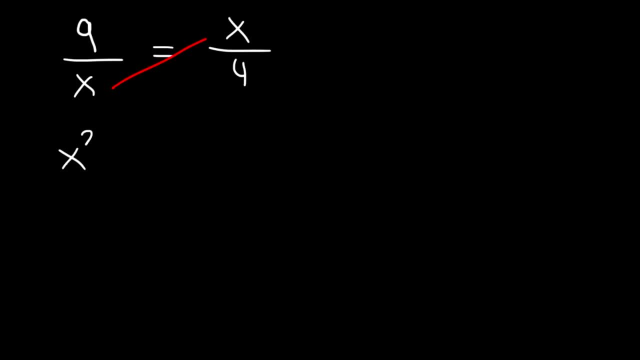 Let's cross multiply. X times X is X squared. And 9 times 4 is 36. So, all we need to do is take the square root of both sides. The square root of 36 is plus or minus 6. So, there's two answers, positive 6 and negative 6. 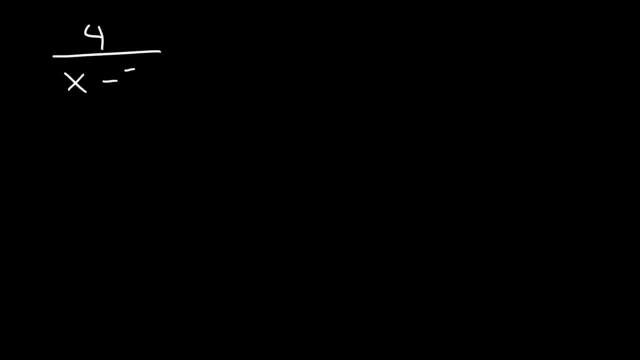 Now, what about this one? 4 divided by X minus 3. And let's say that's equal to 9 over X plus 2. 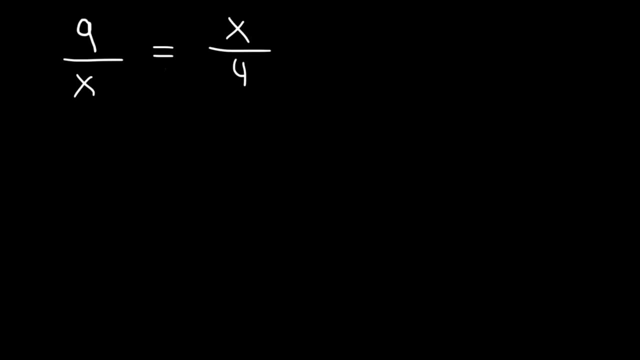 x times x is x squared, And 9 times 4 is 36.. So, once again, two fractions separated by an equal sign: X times x is x squared, And 9 times 4 is 36.. So all we need to do is: 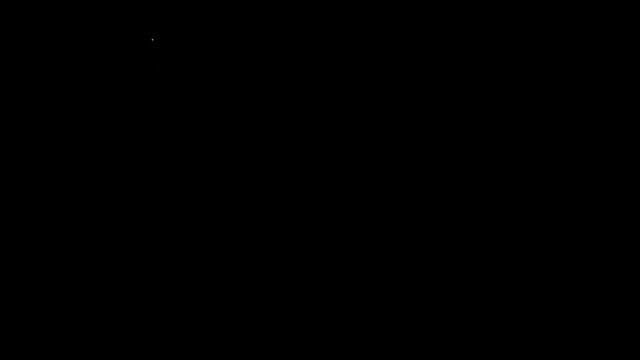 take the square root of both sides. The square root of 36 is plus or minus 6, both answers Positive 5 and negative 6.. 4 divided by x minus 3.. Now what about this one? 4 divided by x minus 3.. 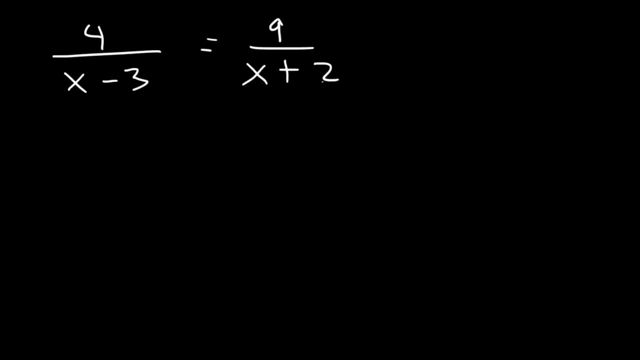 9 over x plus 2, so for this problem as well, cross multiply. so 4 times x plus 2, that's 4x plus 8, and then 9 times x minus 3, that's 9x minus 27, so let's: 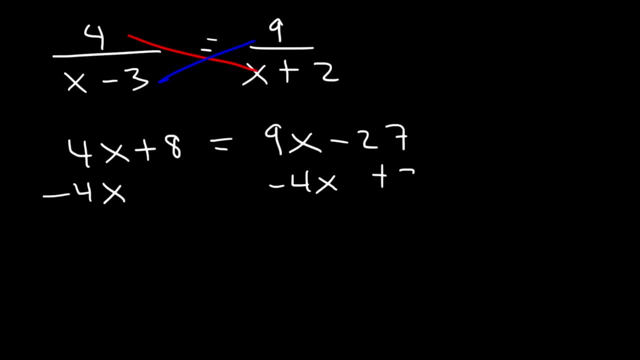 subtract both sides by 4x and let's add 28- I mean not 28, but rather 27- to both sides. 8 plus 27, that's 35. 9 minus 4 is 5. so all we need to do now is divide by 5. 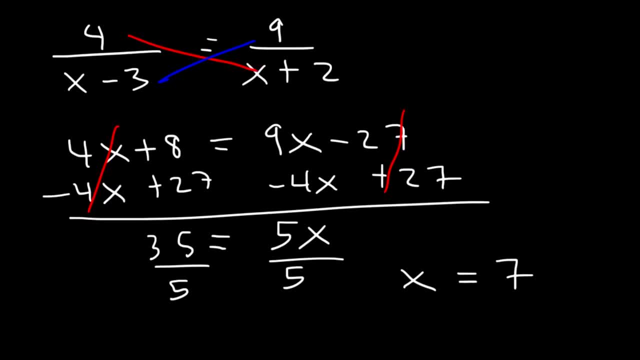 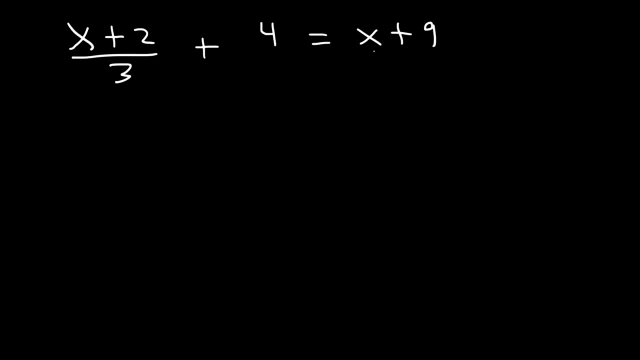 35 divided by 5 is 7, so X is equal to 7. now let's say that we have X plus 2 divided by 3 plus 4, and let's say that's equal to X plus 9 divided by 3 plus 4. and let's say that's equal to x plus 9 divided by 3 plus 4. 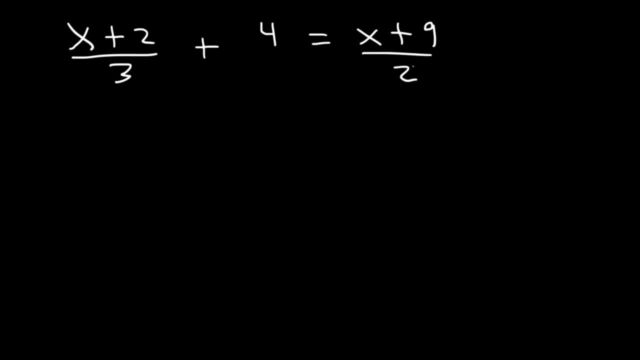 divided by 2, find the value of X. the least common multiple of 2 and 3 is 6. so let's multiply everything by 6 to get rid of the fractions. 6 divided by 3 is 2. now let's multiply 2 by X plus 2 and that's going to be 2x plus 4, now 4 times. 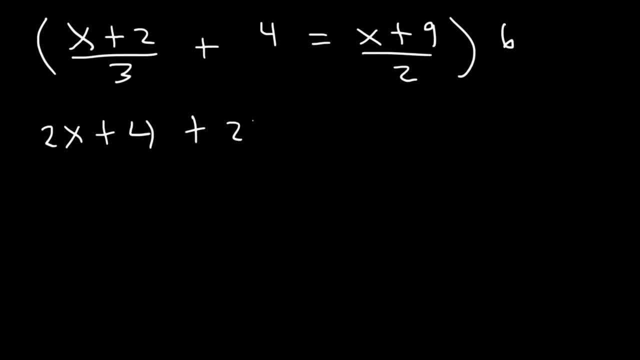 6 is 24, and 6 divided by 2 is 3, and 3 times x plus 9, that's going to be 3x plus 27. so now let's combine 4 and 24, which is 28. now let's subtract both sides by 2, X and also by 27. 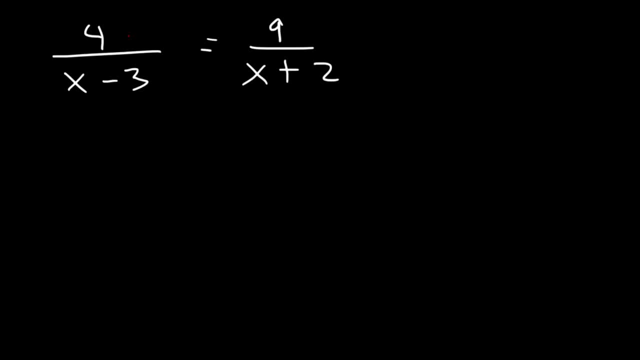 So, for this problem as well, cross multiply. So, 4 times X plus 2, that's 4X plus 8. And then 9 times X minus 3, that's 9X minus 27. So, let's subtract both sides by 4X. And let's add 28, I mean, not 28, but rather 27 to both sides. 8 plus 27, that's 35. 9 minus 4 is 5. So, all we need to do now is divide by 5. 35 divided by 5 is 7. So, X is equal to 7. 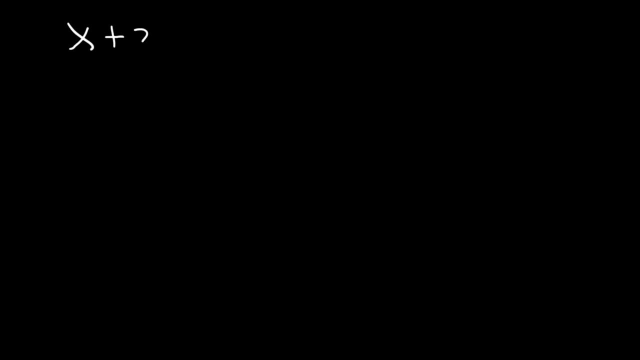 Now, let's say that we have X plus 2 divided by 3 plus 4. And let's say that's equal to X plus 9 divided by 2. Find the value of X. The least common multiple of 2 and 3 is 6. So, let's multiply everything by 6 to get rid of the fractions. 6 divided by 3 is 2. Now, let's multiply 2 by X plus 2. And that's going to be 2X plus 4. 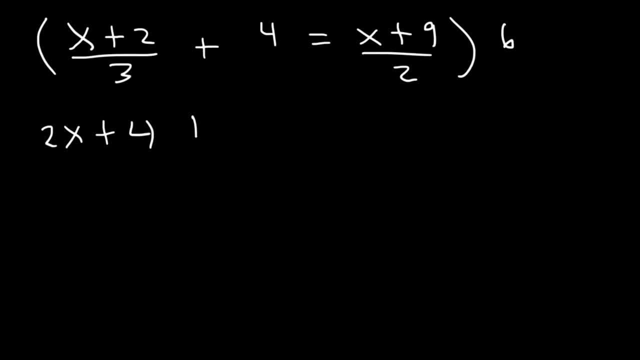 Now, 4 times 6 is 24. And 6 divided by 2 is 3. And 3 times X plus 9. That's going to be 3X plus 27. 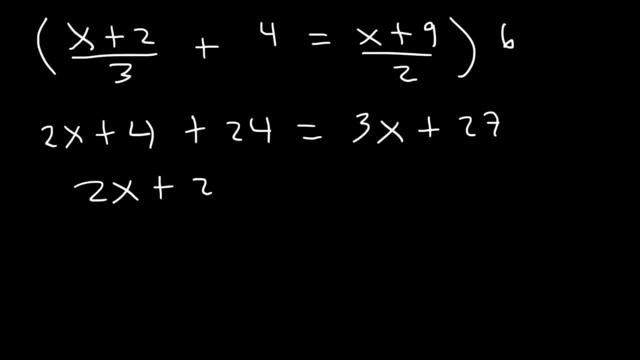 So, now let's combine 4 and 24, which is 28. Now, let's subtract both sides by 2X. 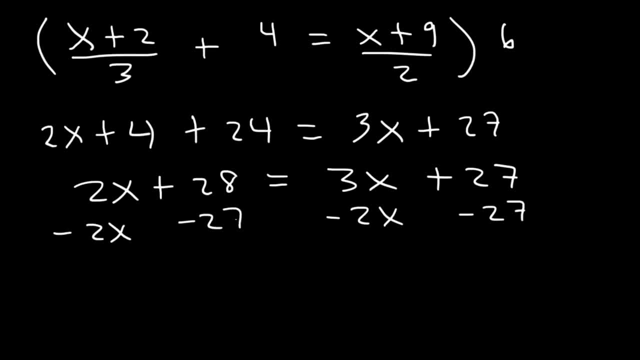 And also by 27. 28 minus 27 is 1. 3X minus 2X is X. So, therefore, X. Is equal to 1. Here's the next problem. 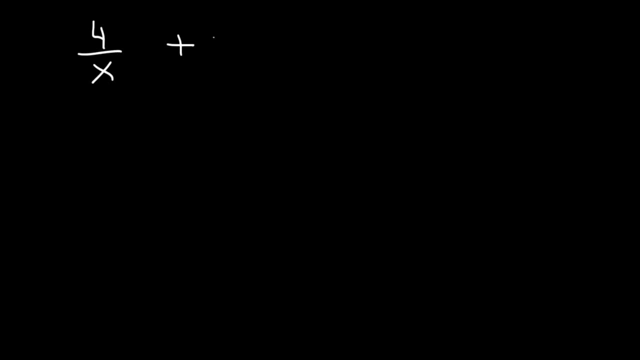 4 divided by X plus 8 divided by X plus 2. Let's set that equal to 4. Find the value of X. 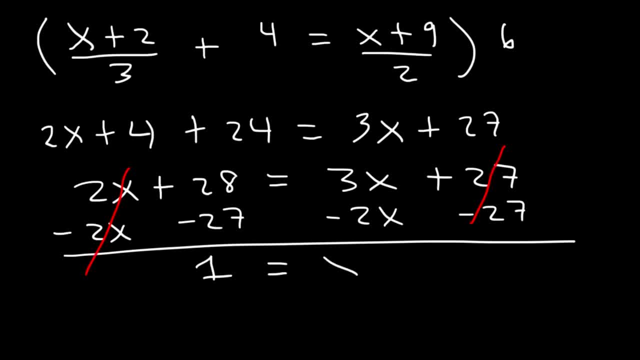 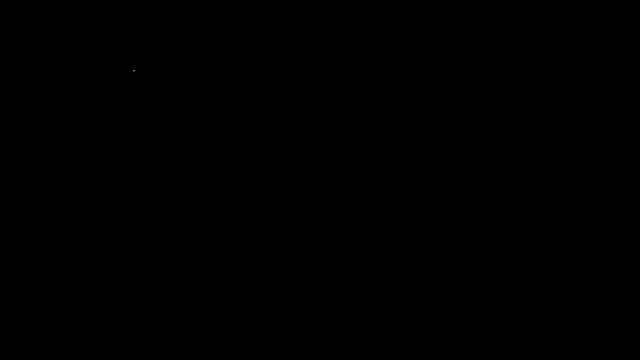 28 minus 27 is 1. 3 X minus 2. X is X. so therefore x. x is equal to 1.. Here's the next problem: 4 divided by x plus 8 divided by x plus 2.. Let's set that equal to 4. Find the value of x. 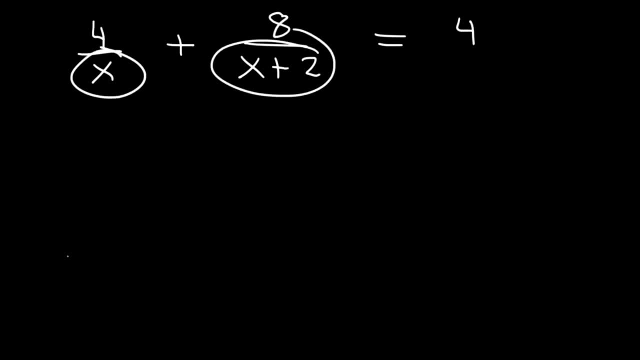 So in this case the common denominator is x times x plus 2.. If we multiply 4 over x by x, x plus 2, the x variables will cancel, And so that's going to leave behind 4 times x plus 2, which, if we distribute 4, it's going to be 4x plus 8.. 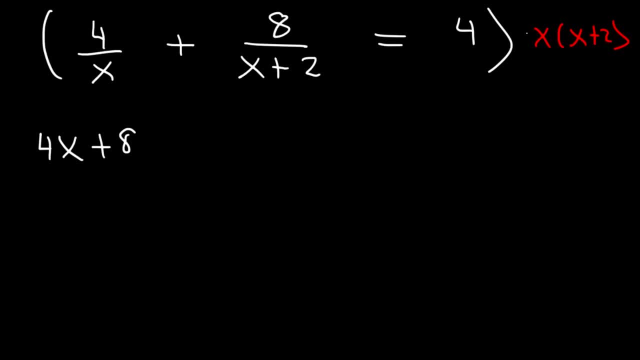 Now x plus 2 will cancel, leaving behind x times 8, or simply 8x. And then here we'll have 4 times x times x plus 2. Which is 4x, x plus 2. Now we can add 4x and 8x. That's going to be 12x. 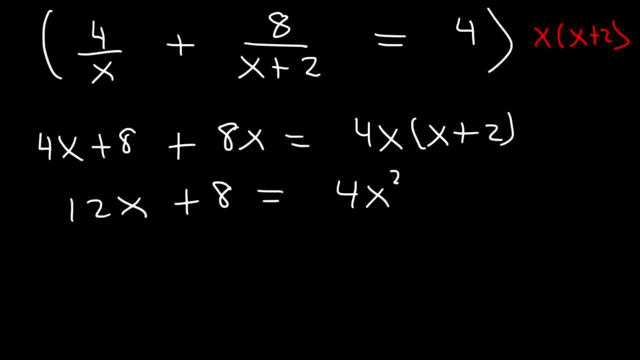 And now let's distribute the 4x. 4x times x is 4x squared, 4x times 2 is 8x. Everything on the left side. let's move it to the right side. So instead of having positive 12x on the left side, it's going to be negative 12x on the right side. 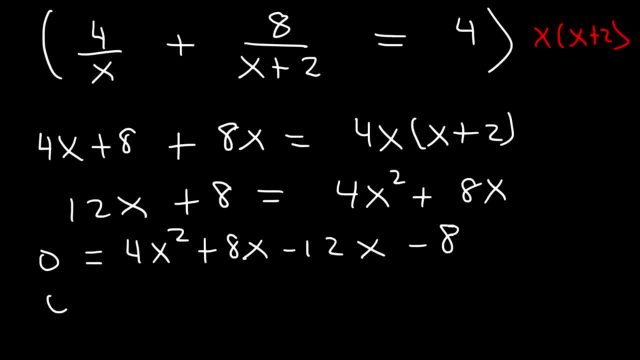 And 8 is going to change to negative 8.. Now let's combine like terms: 8x minus 12x is negative 4x. So now what we need to do is factor. We can take out a 4.. 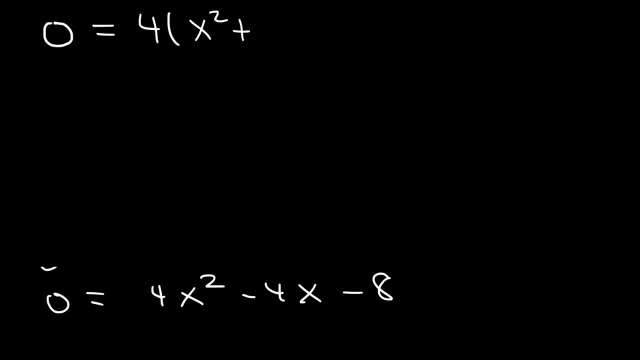 And this will leave us with x squared minus x instead of plus x Minus 2.. Now two numbers that multiply to negative 2 but add to negative 1. It's going to be a negative 2 and positive 1.. 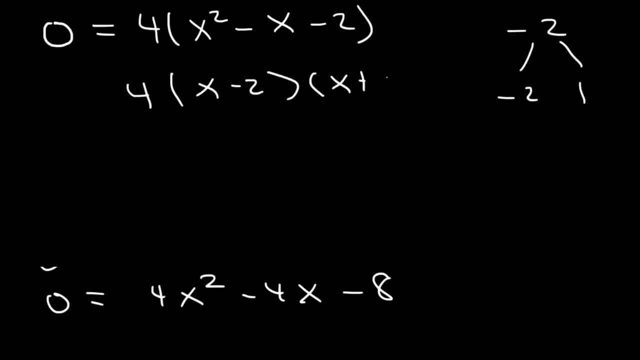 So it's going to be x minus 2 times x plus 1.. So if we set each factor equal to 0, we can see that x is equal to 2 and x is equal to negative 1.. And so that's going to be the answer to the problem. 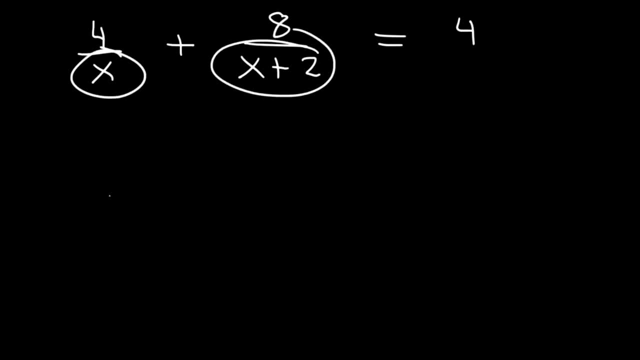 So, in this case, the common denominator is X times X plus 2. So, if we multiply 4 over X by X, X plus 2, the X variables will cancel. And so, that's going to leave behind 4 times X plus 2, which, if we distribute 4, is going to be 4X plus 8. 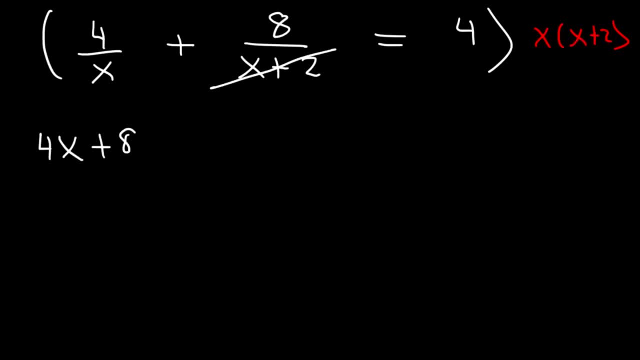 Now, X plus 2 will cancel, leaving behind X times 8, or simply 8X. So, that's going to leave behind 4 times X plus 2. And so, that's going to leave behind 4 times X plus 2. And so, that's going to leave behind X times 8, or simply 8X. And here we'll have 4 times X times X plus 2. And then here we'll have 4 times X times X plus 2. Which is 4X X plus 2. 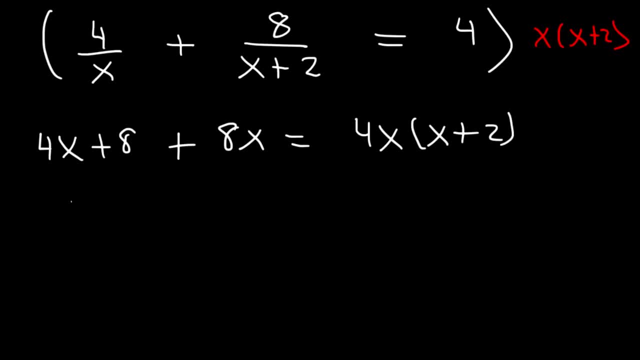 Now, we can add 4X and 8X. That's going to be 12X. And now, let's distribute the 4X. 4X times X is 4X squared. 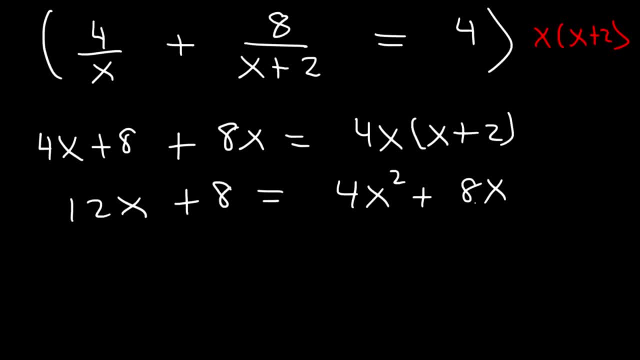 4X times 2 is 8X. Everything on the left side, let's move it to the right side. 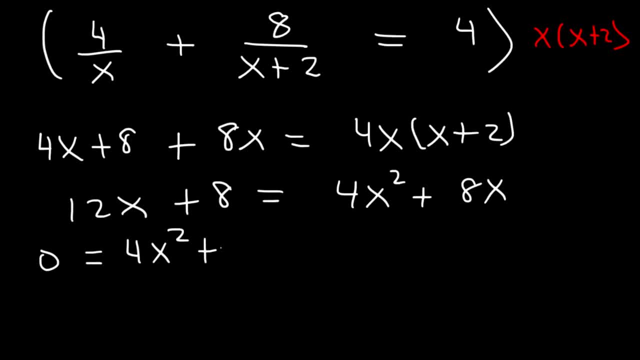 So, instead of having positive 12X on the right side, this will be greater than positive 2X times X squared. left side, it's going to be negative 12x on the right side. And 8 is going to change to negative 8. Now let's combine like terms. 8x minus 12x is negative 4x. So now what we 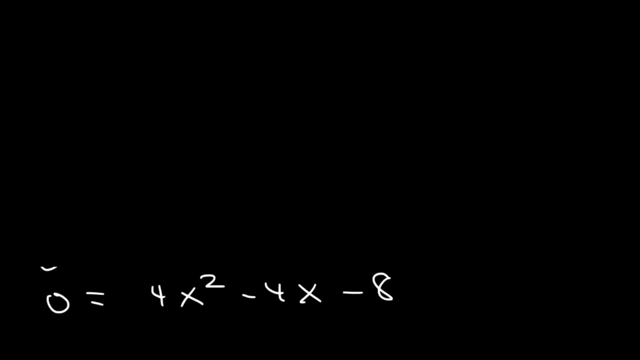 need to do is factor. We can take out a 4. And this will leave us with x squared minus x instead of plus x. Minus 2. Now two numbers that multiply to negative 2 but add to negative 1 is going to be a negative 2 and positive 1. So it's going to be x minus 2 times x plus 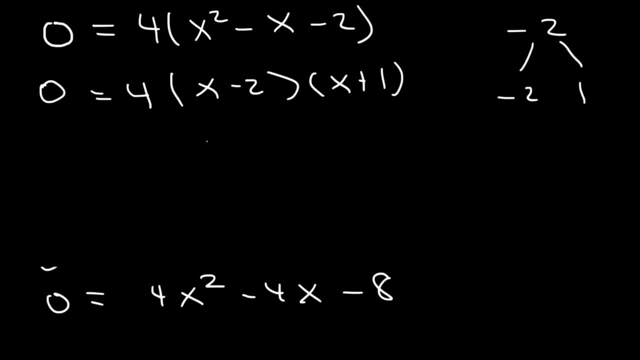 1. So if we set each factor equal to 0, we can see that x is equal to 2 and x is equal to negative 1. And so that's going to be the answer to the problem. 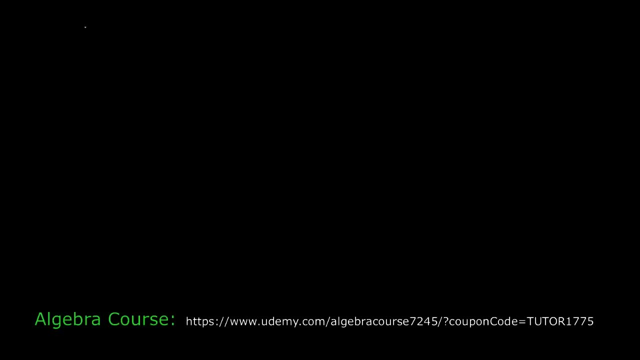 Now let's try the last example. 5, or rather, take that back, not 5, x over x plus 5 minus 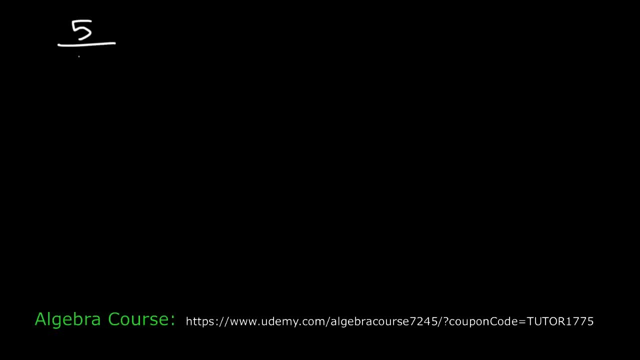 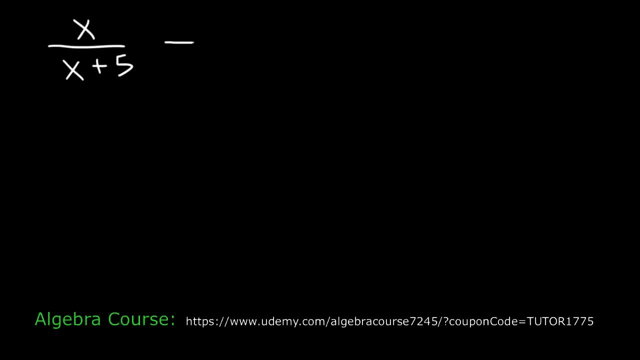 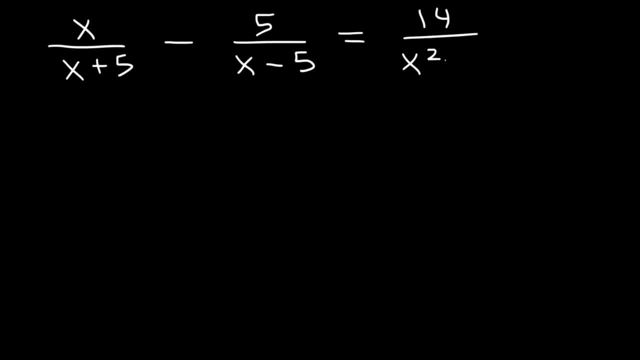 Let's say that's equal to 14 over x squared minus 25.. Go ahead and find the value of x Now. what we should do first is factor x squared minus 25. And that's going to be x plus 5 times x minus 5.. 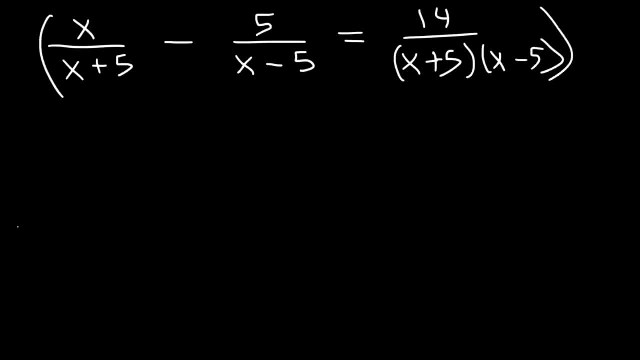 Now we need to clear away the value of x, all fractions. So let's multiply the top. well, let's multiply both sides, the left side and the right side, by x plus 5 times x minus 5, the common denominator. So if we take this: 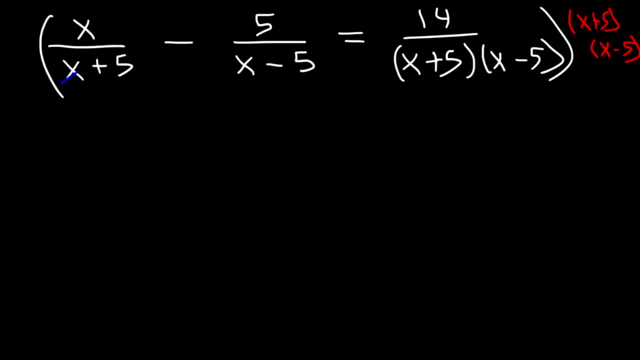 fraction and multiply it by these two, we can see that x plus 5 will cancel, leaving behind x times x minus 5.. Now if we take the second fraction and multiply it by those two, the x minus 5 term will cancel, leaving behind 5 times x plus 5.. And then x plus 5 will. 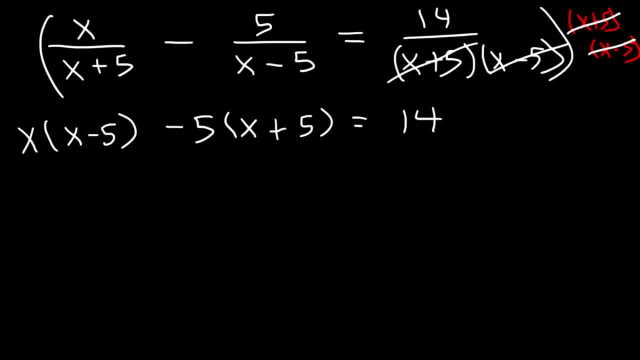 cancel leaving behind x times x minus 5.. And then x plus 5 will cancel leaving behind. x minus 5 will cancel leaving 14.. So now let's distribute x times x minus 5. That's x squared minus 5x. And if we distribute the negative 5, it's going to be negative 5x minus.